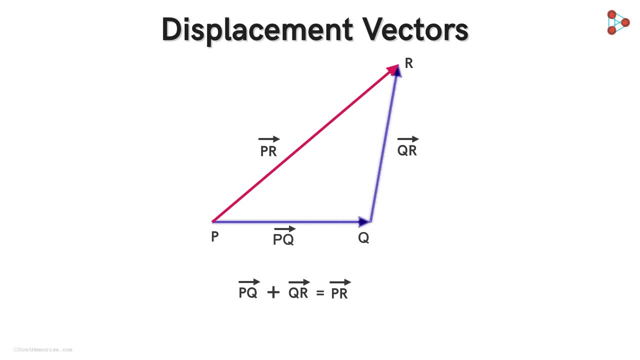 That is, from P to Q and then from Q to R. Now we take the third side of the triangle Here. instead of taking it in the same order, that is, from R to P, we take it in the opposite order: P to R. 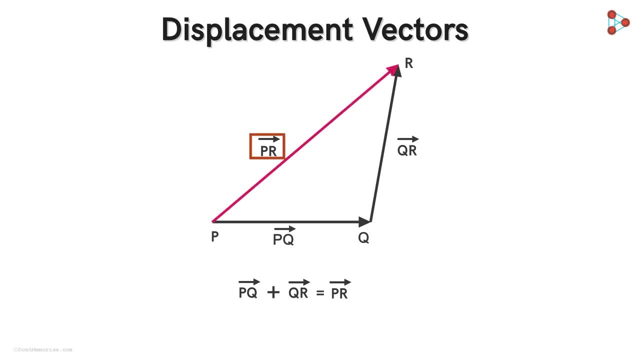 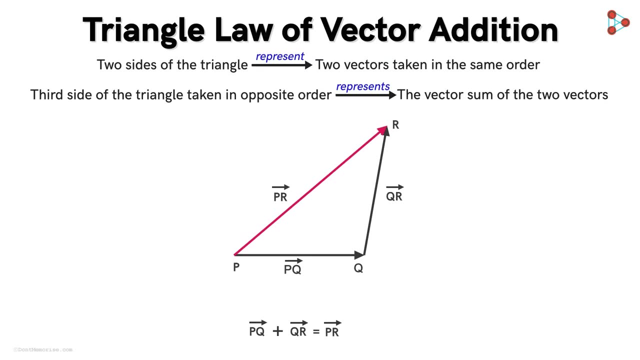 Then the resultant vector PR, will represent the vector sum of the two vectors, both in magnitude and direction. This is known as the triangle law of vector addition. Take a moment and have a look at this Now. by applying this law, we can add any two vectors. 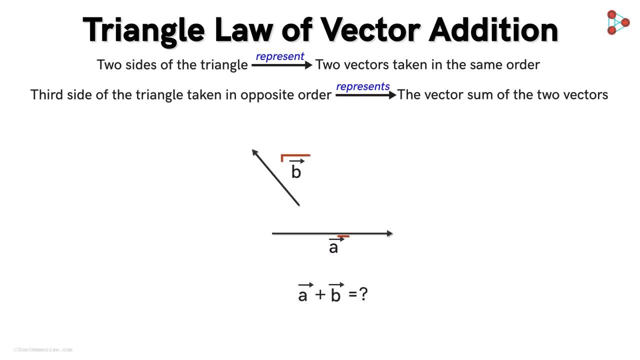 Suppose we have to add these two vectors, A and B. So for this first we need to position the two vectors such that the initial point of one vector coincides with the terminal point of the other vector. So we move the vector B parallel to its position. 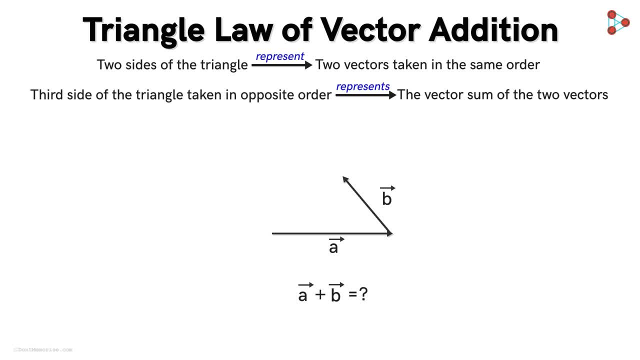 without changing its magnitude and direction, And place it such that the initial point of vector B coincides with the terminal point of vector A. Now notice that these three points, A, B and C, form a triangle, So according to the triangle law of vector addition, 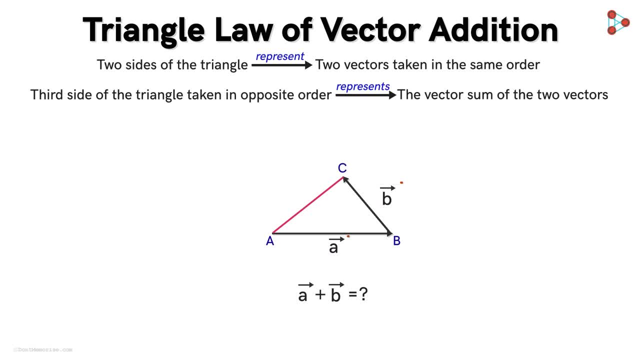 the vector sum of these two vectors will be the third side of the triangle, A, B, C, such that its initial point and that of vector A coincide and its terminal point and that of vector B coincide. We write it as this: So in this way, by applying the triangle law of vector addition, 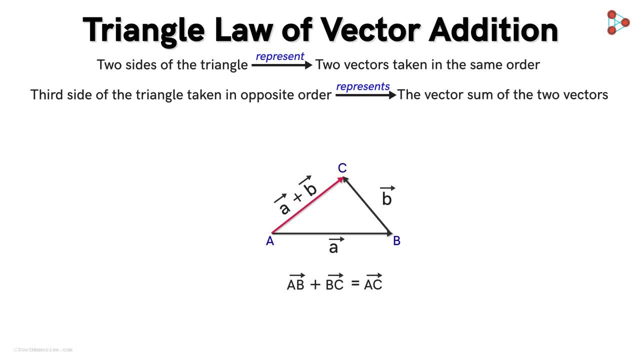 we can find the vector sum of two vectors. Here we can find the magnitude and the direction of the vector A- C by using geometric properties of the triangle A, B, C. But it's a little difficult, Hence we will see another, easier method for this in our upcoming videos. 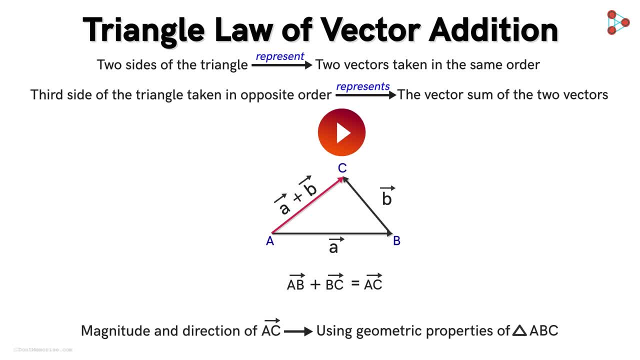 Here. we just need to understand what does the addition of vectors mean intuitively? Now suppose, instead of two vectors, we want to add these four vectors. What will the vector sum be? Can you apply this law here? Right, It will be this vector whose initial point will be the initial point of vector A.